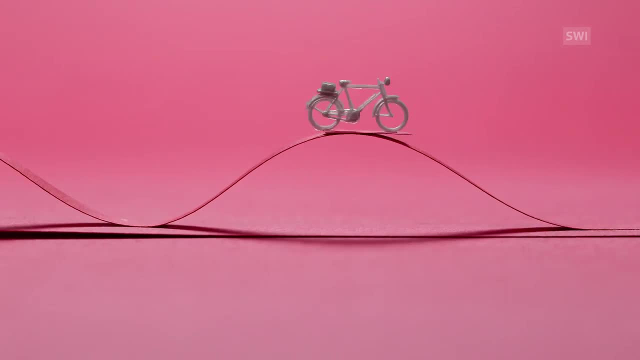 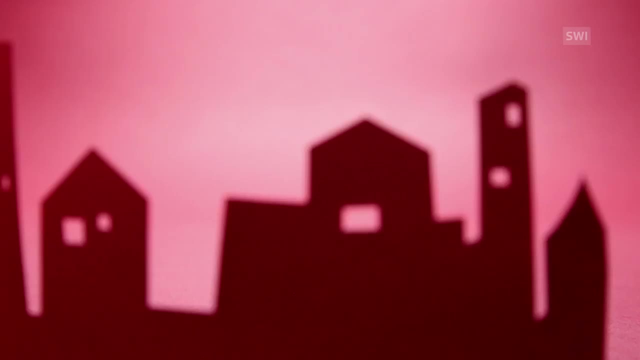 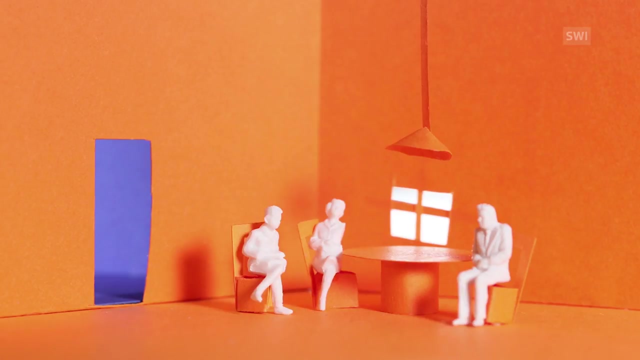 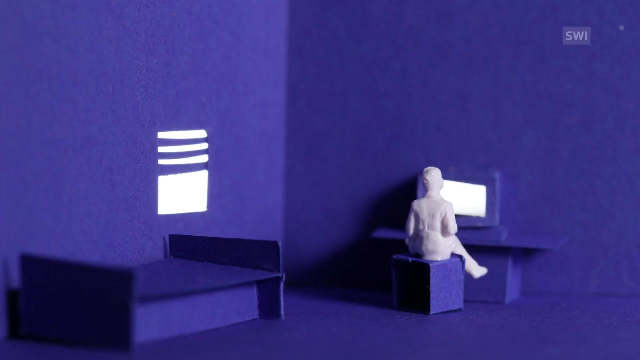 He collects signatures for a proposal to introduce more bike lanes in his town. Max became involved in politics through his parents- His mum's a local parliamentarian, so political issues were often discussed at home. He also finds a lot of information online and discusses topics with friends via social media. 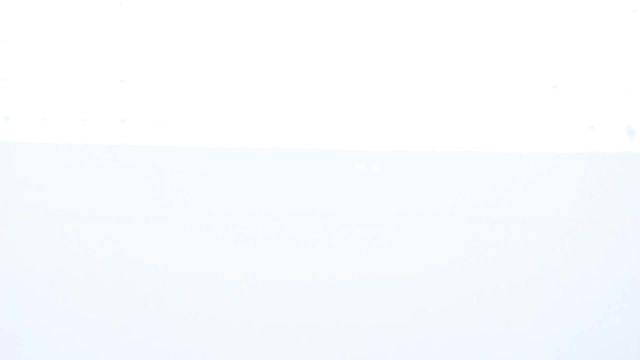 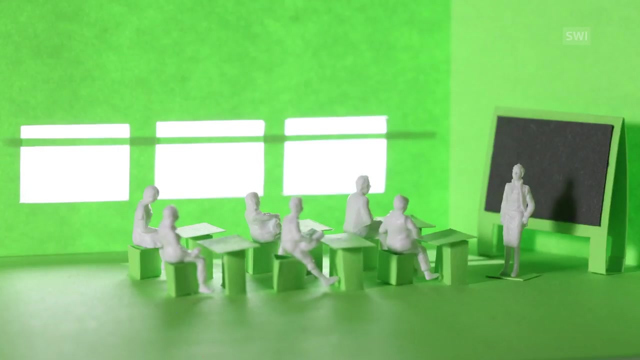 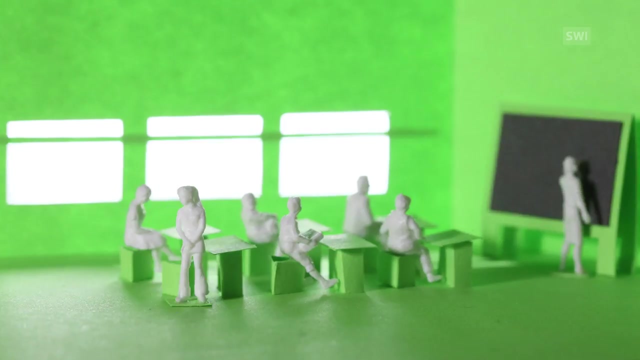 You could say Max gets his civic education from his family, His friends and social media. Others, like Tamara, learn about it at school. Tamara's parents were immigrants to Switzerland. They didn't know much about the political system here, and learning all about it didn't grab Tamara at first. 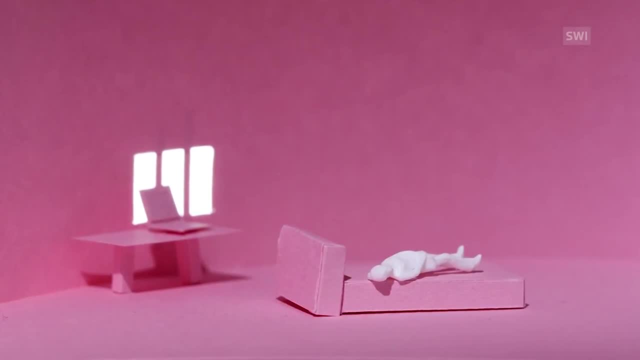 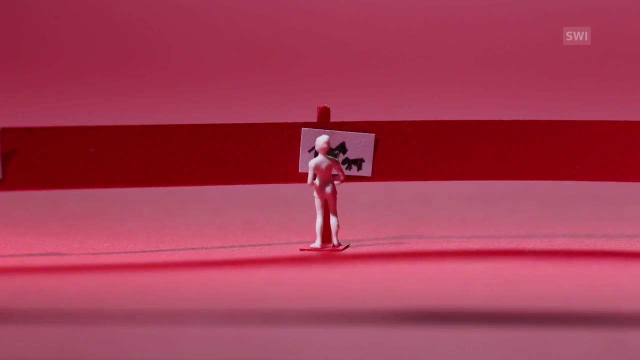 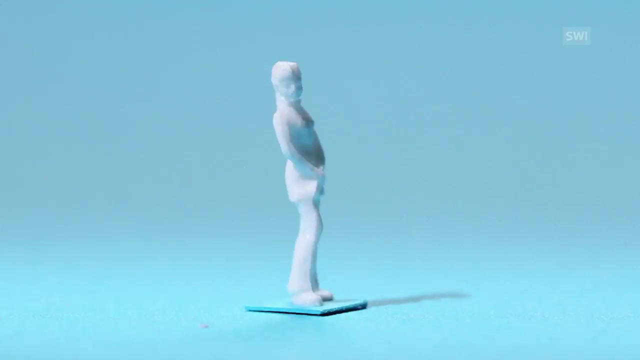 So what changed her mind? One day, her class was asked to propose things that could be improved. Tamara was especially interested in giving more rights to immigrants. She eventually became Swiss. Now she's in her late thirties and exercises her right to vote. 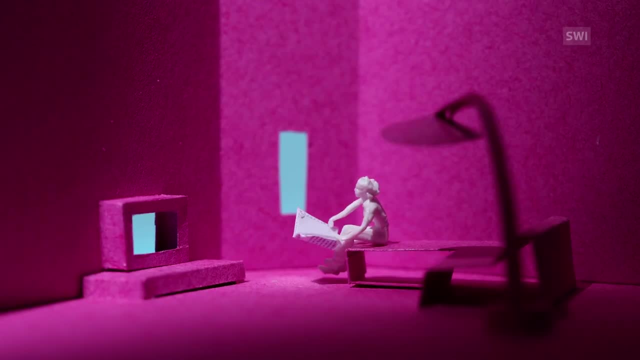 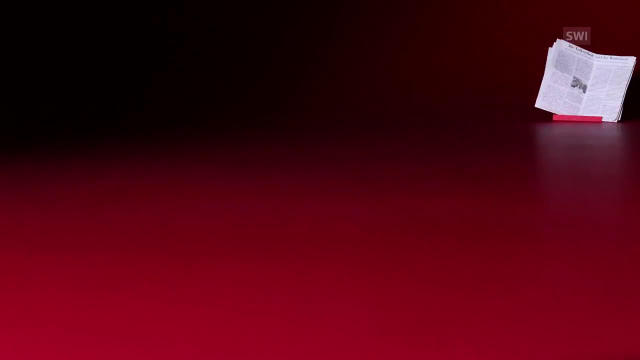 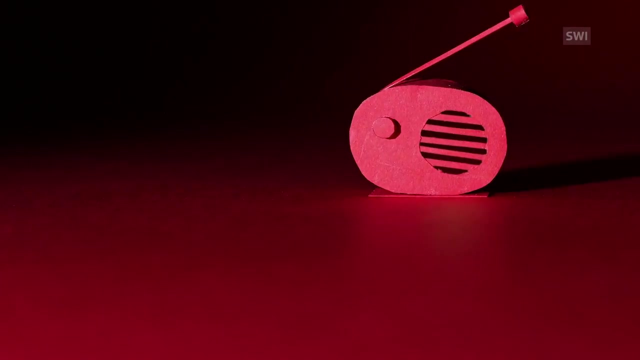 She finds out about votes coming up via the media. That is why the media is often referred to as the Fourth Estate. The press has no direct say in a country's politics, but has a large impact on public opinion. Civic education can also come from political parties. 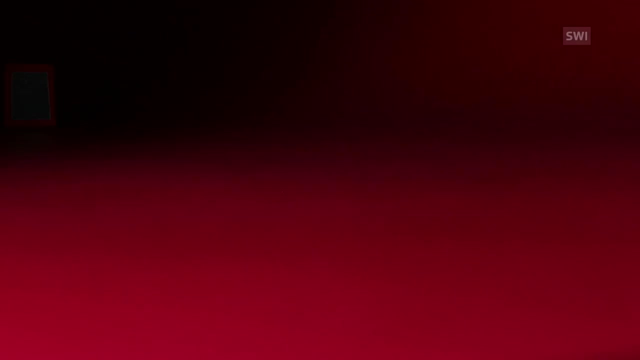 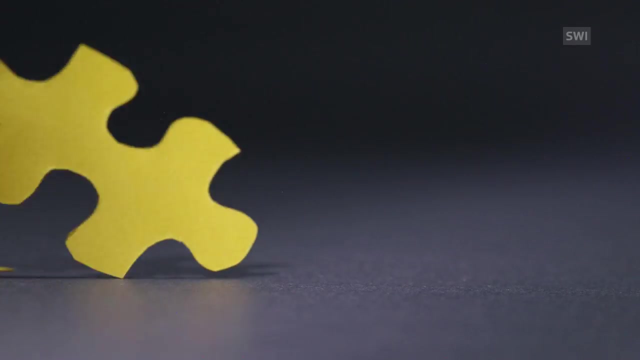 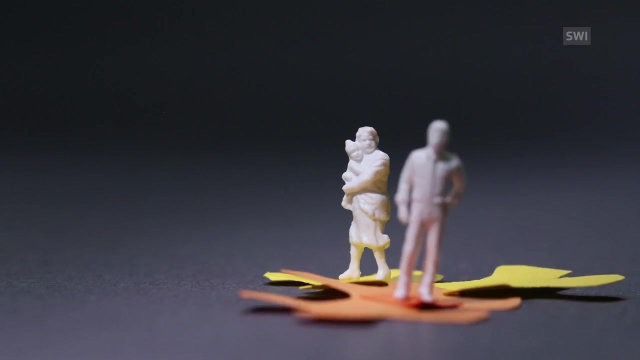 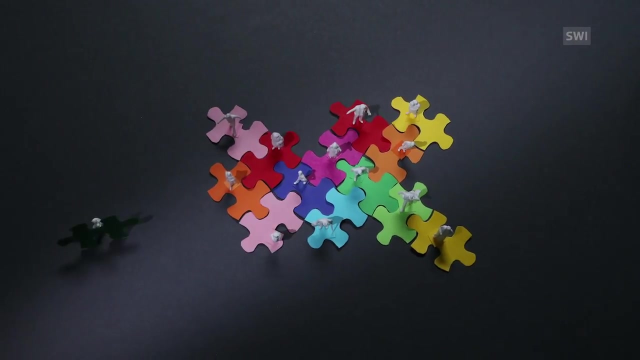 when they pass on information to citizens to help them make up their minds. Why is knowing about rights and democracy important? Democracy only works if people know about the rules and play along. Many democracies suffer from poor participation due to poor civic education, And there's room for improvement in Switzerland, too. 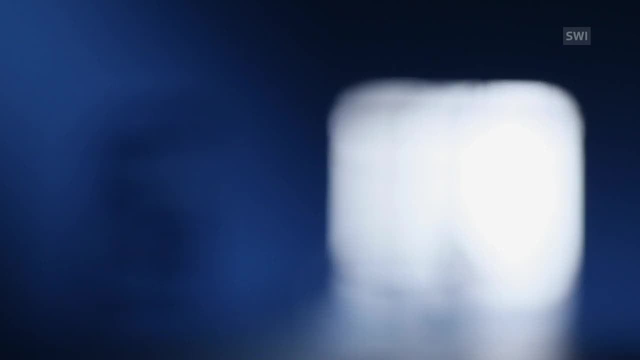 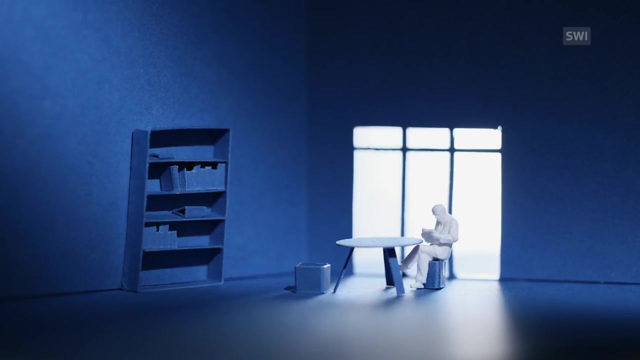 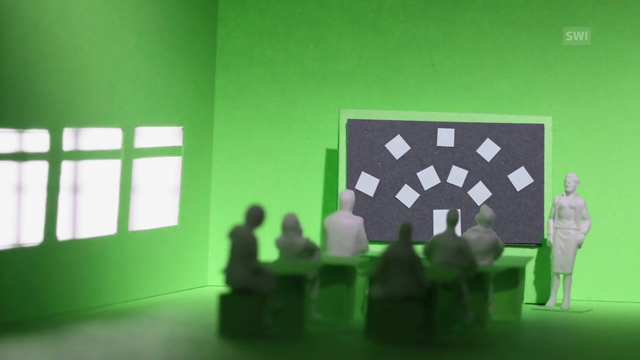 There are many reasons why people don't bother to cast their votes. The issues at stake may be too complex to understand, Or they just don't think their vote will make a difference. Surveys show that the Swiss believe civic education is the best way to improve democracy.